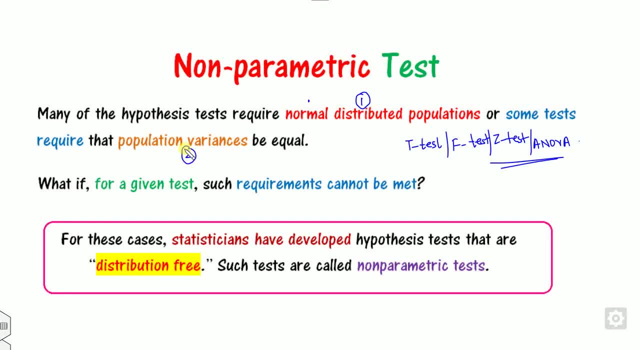 variances are equal. But what will happen if such requirements cannot be met? If such requirements cannot be met, then what will happen? If such requirements cannot be met, then what will happen If such requirements cannot be met? it means the population may or may not be the normal. 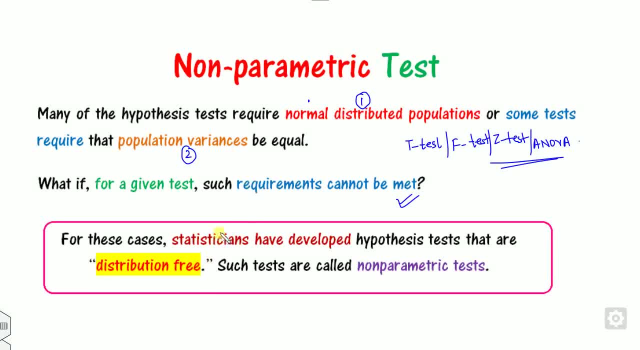 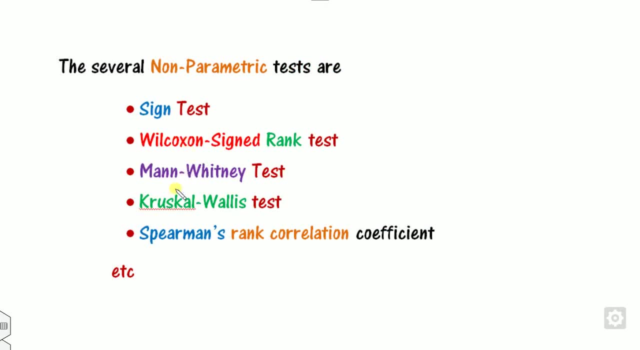 distribution. So in order to handle this, the statisticians have developed the hypothesis testing that is called as the distribution free, and such tests are called as the non-parametric test. So there are the several kind of the testings which are listed as here. Sign Wilkerson Mann. 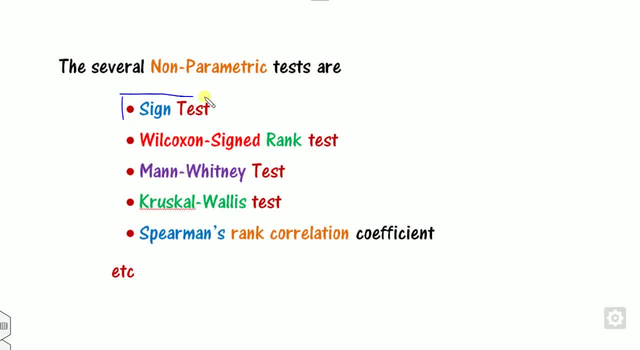 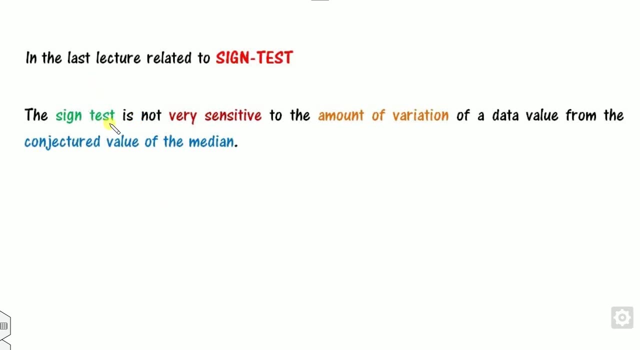 Crucial and so on. So in the last lecture what we have studied is here Now. this today we will discuss about this lecture, that is, the Wilkerson sign rank test. What are the drawback of the sign test? So, first of all, what we see in the last test is the sign test. 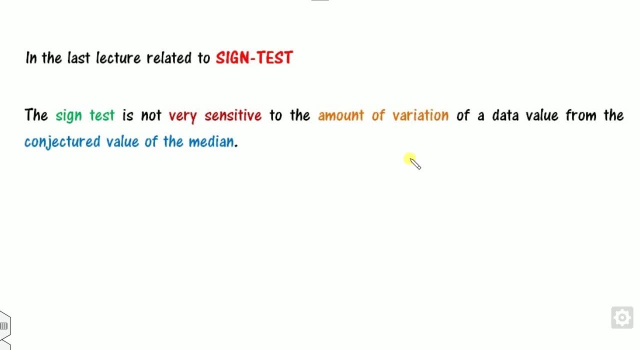 is not very sensitive to the amount of the variation, What we have seen in the last lecture. if you missed the last lecture, you can see the description of this video. You can find easily. the sign test is there. So say, my numbers are here and I want to apply the. 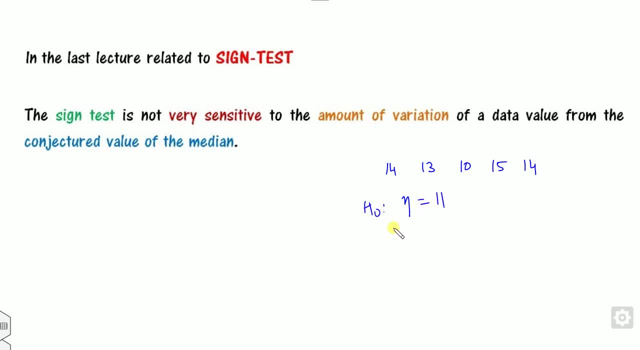 H0 median as, say, is 11, or say you can say okay, 11, and this is not here. So what you can do is you have to subtract 11 and take the positive. negative signs are there according to the divisions. So this is positive and positive. But look at that. if I just replace 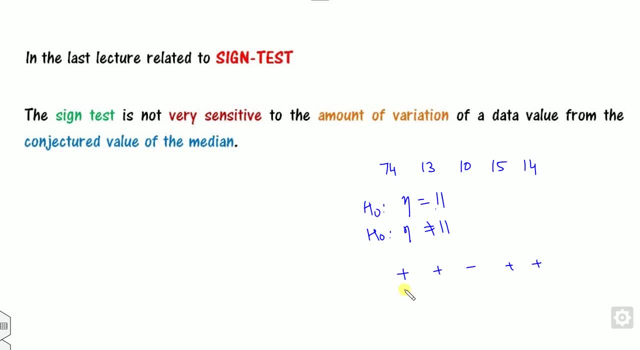 this 14 to be the 74, the sign will remain the same. So that is the most important drawback of this sign test. The sign test is not very sensitive to the amount of the variation. Look at that. the amount of variation of 14 to 3 is 3.. There is a plus of 3.. Here is plus of 4 and here. 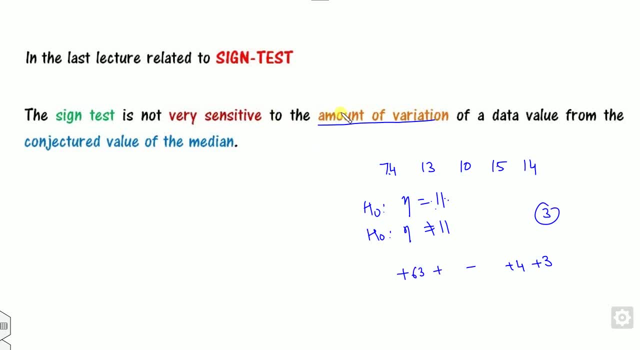 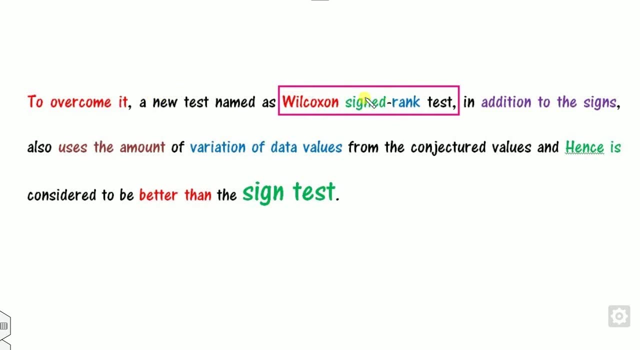 is 60 of 3.. But this is completely independent of them, So it uses whether the numbers are positive or negative, or called as the above and below. So consequently, it will fail in rejecting the null hypothesis H0.. So to overcome this, there is a new, there is a some: the person. 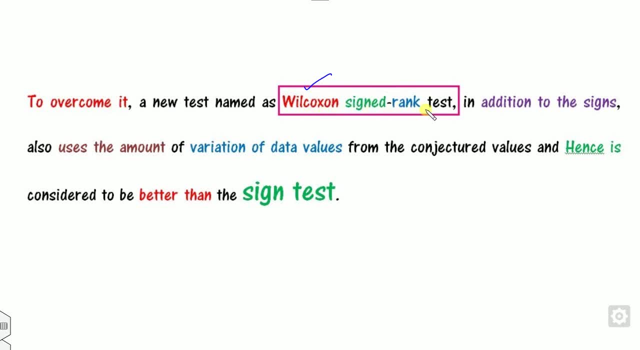 will call will develop. this will call sign rank test, to gap this. So in order to understand this will call sign rank test. I just firstly explain what is the meaning of this sign test and how we can compute the sign rank. So firstly discuss. 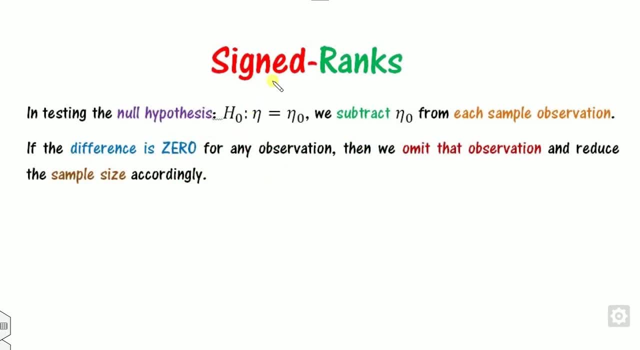 about that rank. I call as the null hypothesis. H 0 is here, we will subtract this quantity, whatever you have written here. if I just write H 0, 5, then you can subtract 5 from each observation and if there is any difference is 0, then we can omit that observation and reduce the sample size. so look, 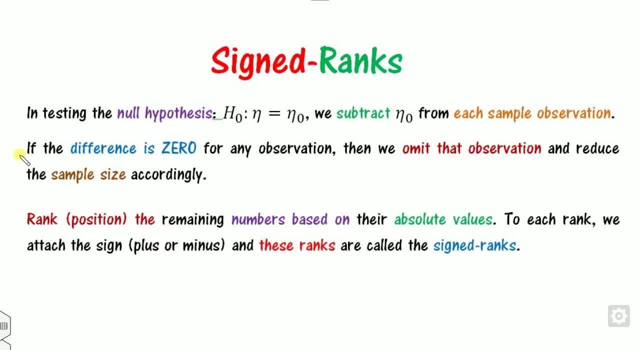 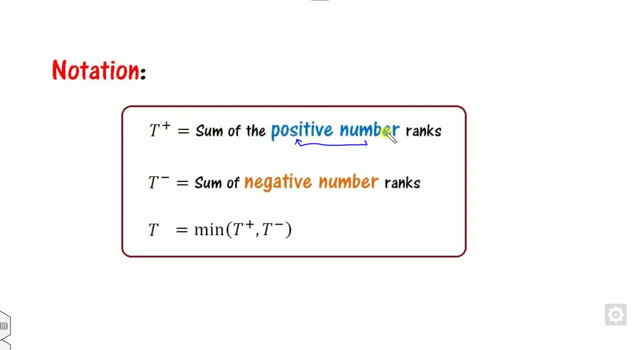 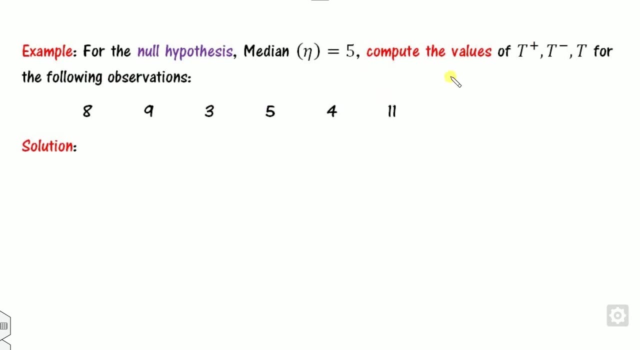 at that. how look at that? so this: I use the notation as: t positive sum of the positive number rank, t negative is the sum of the negative number rank and t is the nothing but minimum among them. so look at this example. you have to compute the t positive, negative and the t for this. 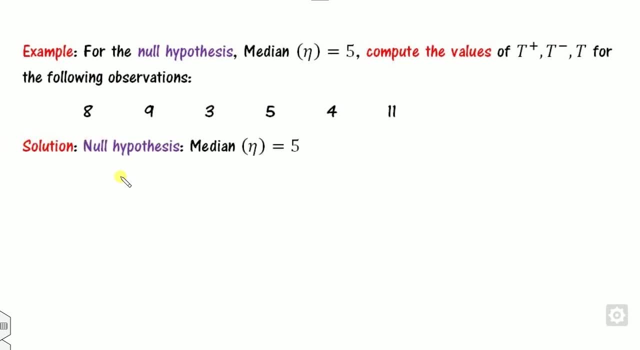 particular problem. so, first of all, what is the null hypothesis is? it is given to 5. subtract 5 from each of the numbers, so you can get 5 8 minus 3, 5, 3, 4 and so on. if you use the sign test here, then what you get is: 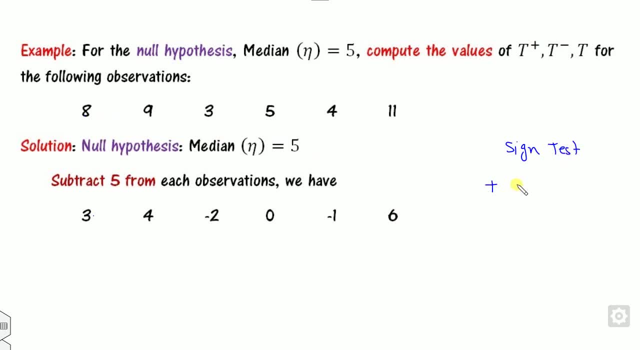 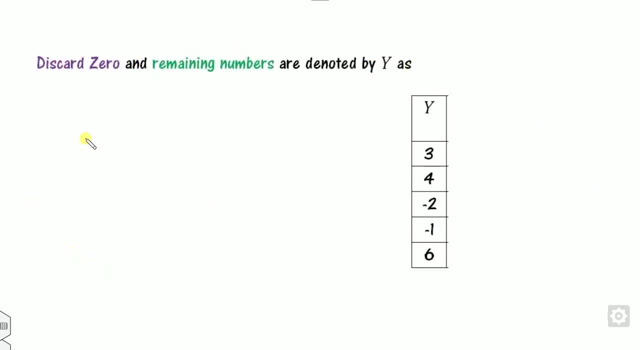 you have to use only the rank 8 minus 5 plus 3 plus 4 minus 2 0 minus positive. okay, so we are not using the sign. so these are there now. check whether there is any 0. yes, so if there is any, 0. 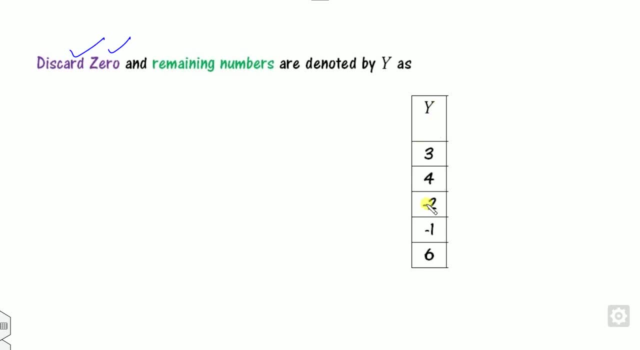 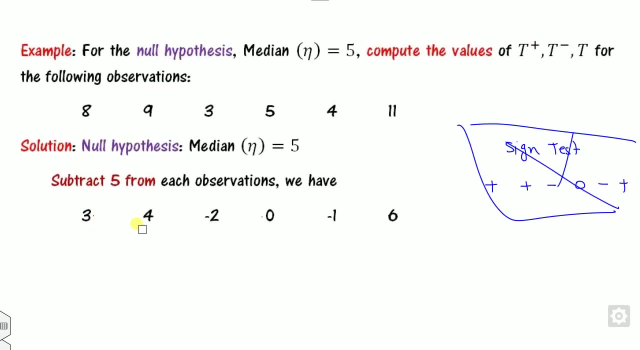 present, you have to discard the 0 and write it as t positive sum of the numbers, and the result is the value of t plus a minus 5, minus 5, minus 4, plus over 0. alright, and then subtract 5 from each other. where is t? 1? because this is sans sign. so how do we have 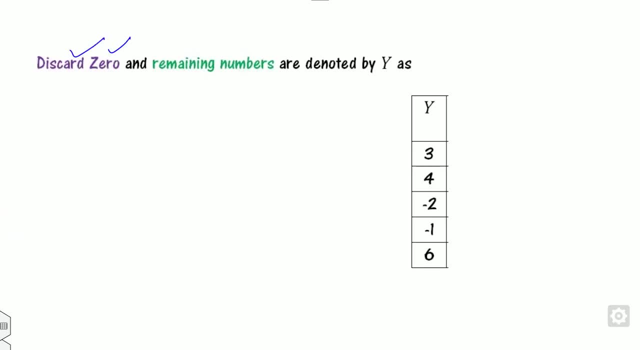 the option to also use this surface line 0. this can be done by putting an function here at 0, because 0 is minus pi by 2 times. I am between 1 and 1, and it should be 0, because you already know that what you will get is on the other side. andひ, for example, means 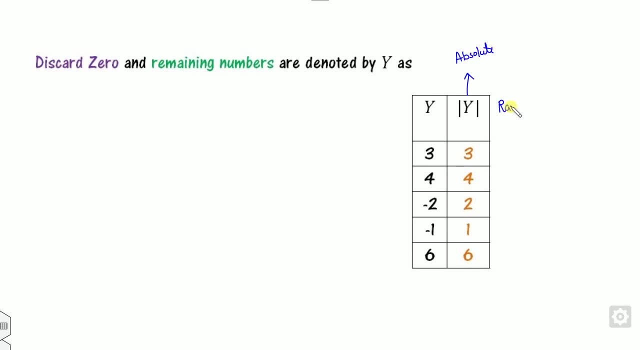 1. that is what is not your own one, so 0. so y is not my own partial number right now. that will then just instead of 0, where is 0? I can just assume that there is 0. okay, if you see here S is x, kaçy in S is x, you really have no choice but to P�. 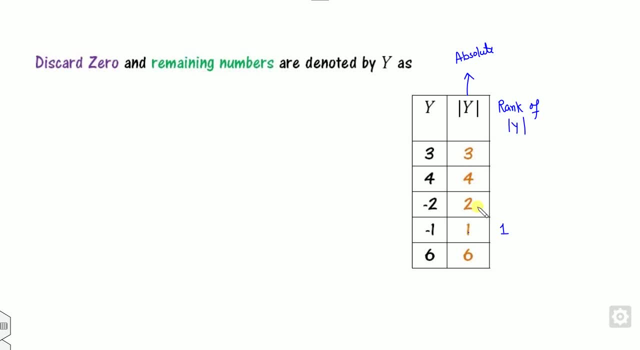 then you leave. so y got you didn't solve the same problem. okay, so we will discuss a Cle ajust here. absolutely the next. you will need to find the ranking of mod y, the position we, So you can take as a 1.. What is the next smallest number is this: 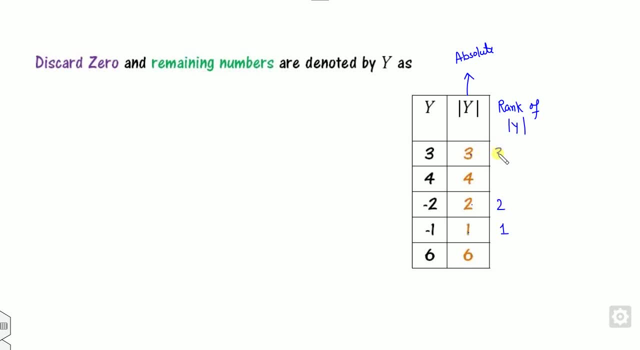 Take as a 2.. What is the next smallest number is 3.. Take as 3.. What is the next smallest number is 4.. What is the next smallest number is 5.. So this is the rank of Y. Okay, 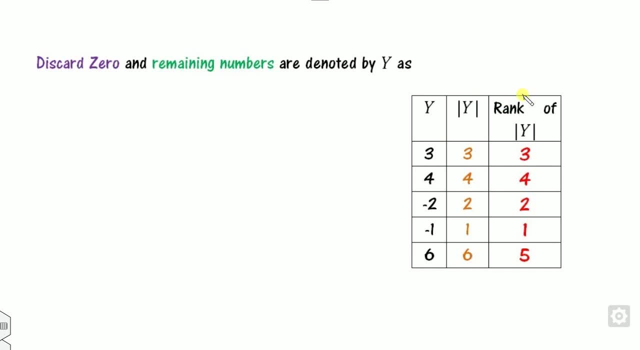 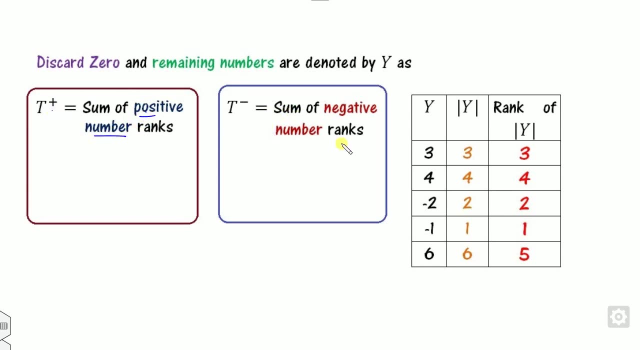 So look at that Now you, once you are taking the rank of this, You have to define the T positive and T negative. What is the T positive is sum of the positive number rank. Look at that. These are number which are the positives. 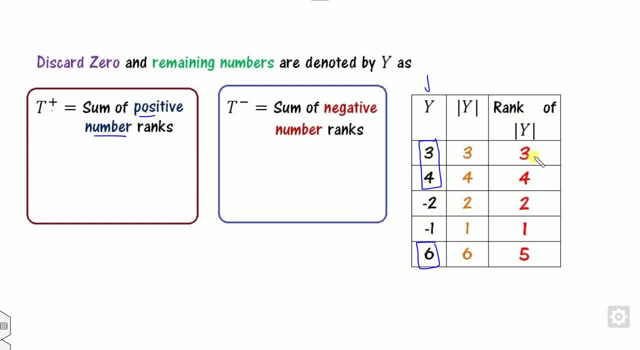 This 2 and this 1.. And what is the rank is 3,, 4 and 5.. So you can take the sum. Look at these 3 quantities are positive. So take the rank of 3,, 4, 5.. 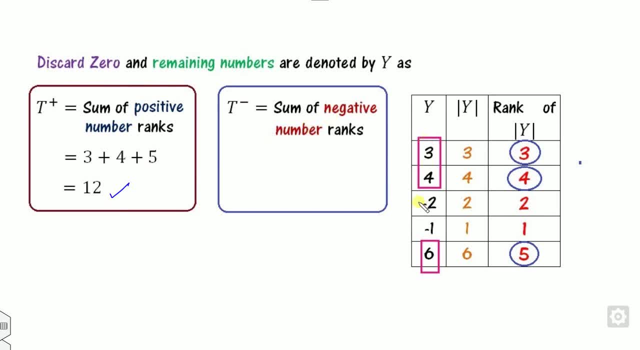 That's a 12. Sum of the negative number, rank Which one are negative, This and this. So you can compute the rank sum rank. That is a 2 plus 1, 3.. Once you compute the T positive and T negative, 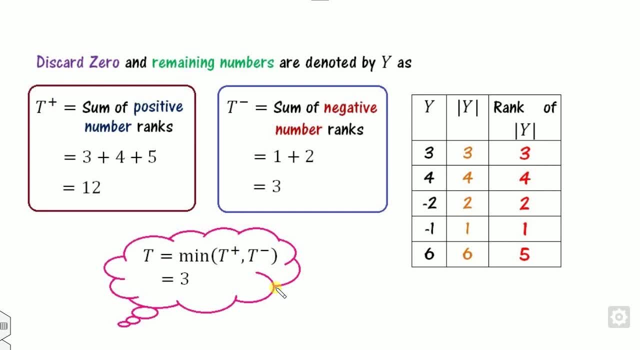 You can find the T as the minimum. So this is the way you can compute the T positive, T negative and T. But look at that. There is a no repetition among them. For example, if I say instead of this, there is a 4.. 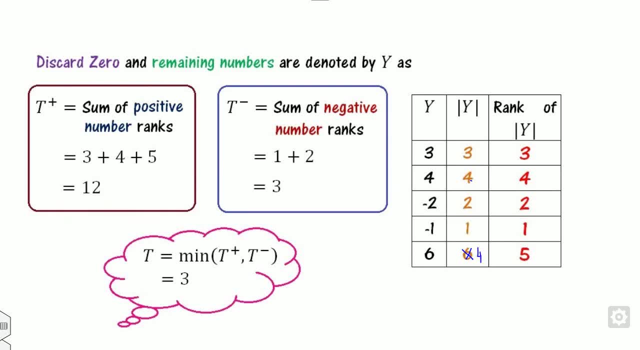 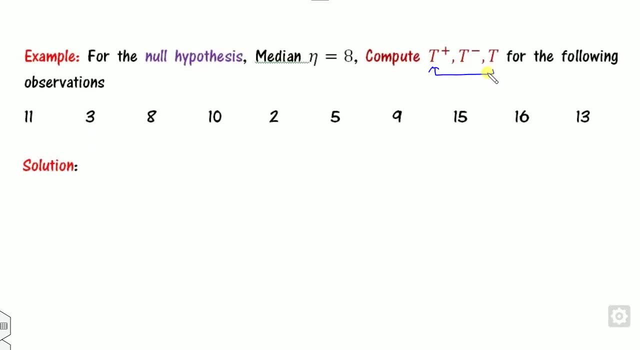 So how you rate them. These and these are same. So, in order to case of the repeated rank, how you solve them. So look at that again. You have to compute these numbers. So what is that? 0 is here, Subtract 8 from the each numbers. 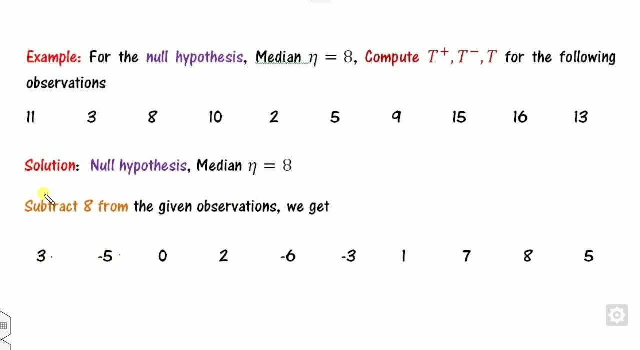 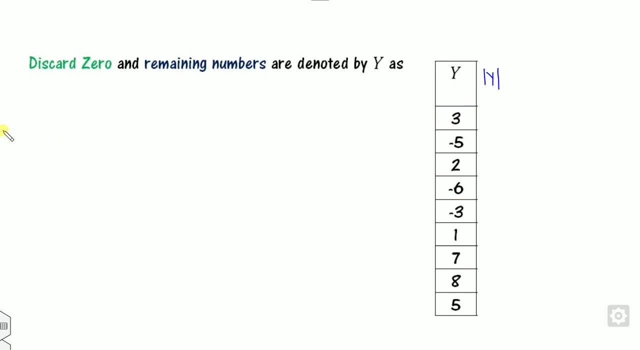 You will get this, this and this And then discard The 0 and write all numbers in the series. Now you can find the mode of y firstly. You will get as here. Now you can firstly rank them. Which is the smallest number is here. 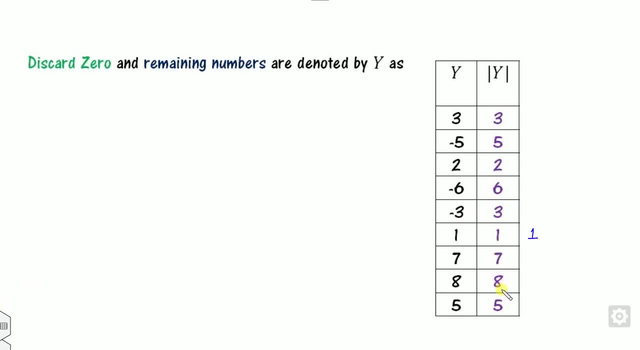 So put them as a 1.. What is the next number is 2.. So this as my 2.. What is the next number is This: and this: both are same. Okay, So it means this is the position of third and fourth. 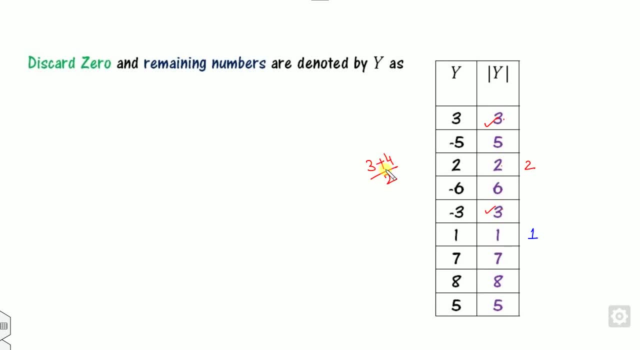 So you can write as 3.. Plus 4 divided by 2, because there are the two numbers. So this is my 3.5.. So this is 3.5.. This is 3.5.. Okay, So this is 1, 2.. 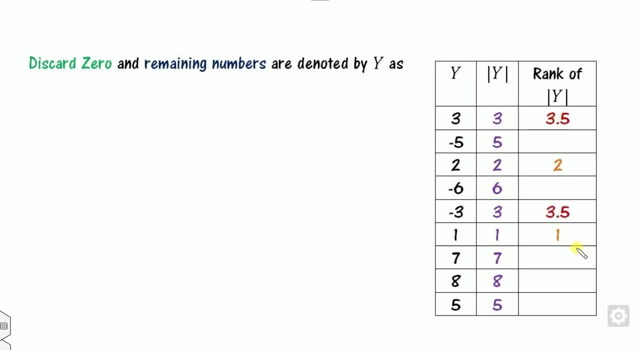 Now both are the same numbers, So you can write this as 3.5, 3.5.. Now look at. the next number is smallest, is 5, 5, 2 times. So what is the position? is we already put up the four numbers: 1, 2, 3, 4.. 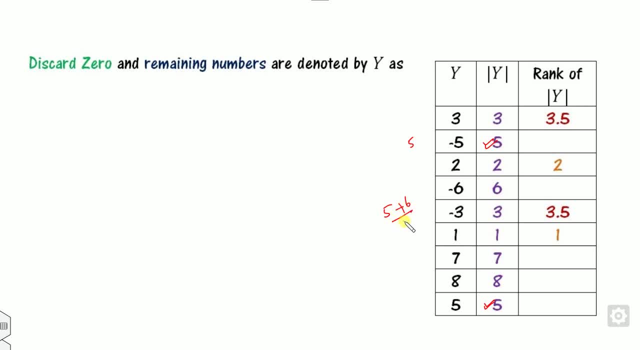 Now this is 5. And 6.. So 5 plus 6 divided by 2 is 5.5.. So you can put as 5.5, 5.5.. Now look at the next number is: this is 6, only 1 times. 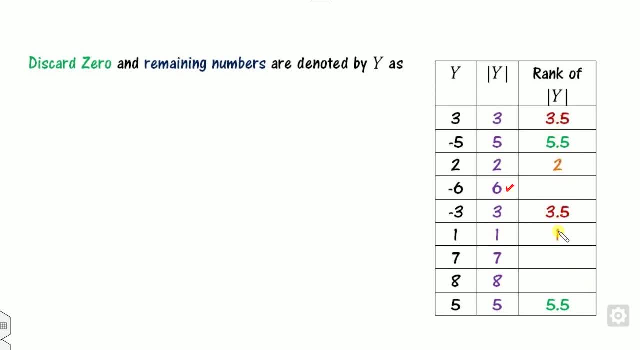 So how many numbers we have put up: 1, 1,, 2,, 3,, 4,, 5, 6.. Now its number is 7.. After that, this is 8 and this is 9 because it occurs only 1 times. 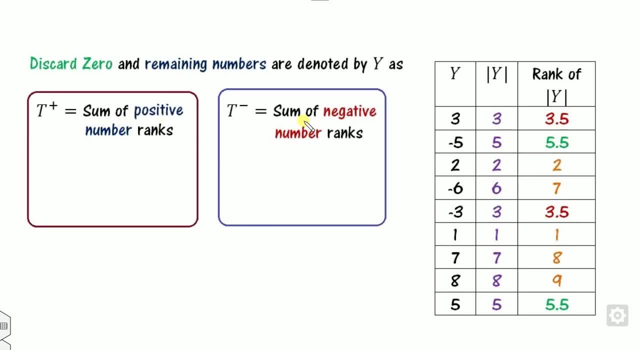 Now, once you complete the rank, you have to define the T positive and T negative. So firstly you define the T positive. Which one numbers are positive, This, this and this? So the corresponding ranks are 3.5,, 2 and these four quantities. 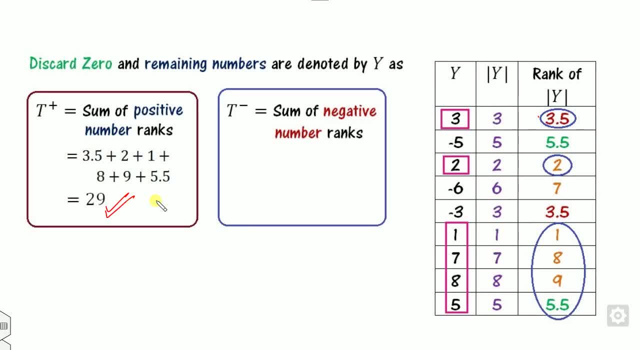 So you have to add them. You will get T positive. What is the T negative is? you can say the meaning of them, or else this is a negative, This is a negative, This is a negative. So you have to find. the numbers are here. 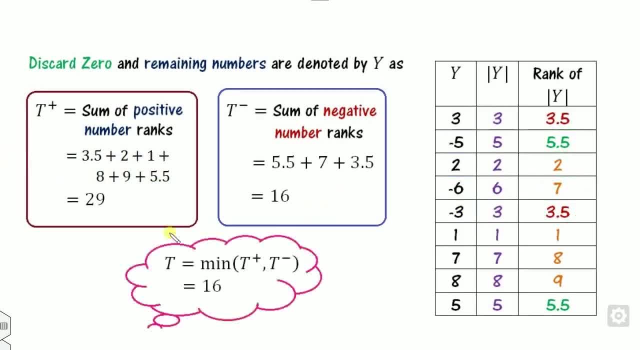 Once you get T positive and T negative, Then we will get the T positive. So you have to find the numbers are here. Once you get T positive and T negative, Then we will define the capital T as 60. So this is the meaning of this signed rank. 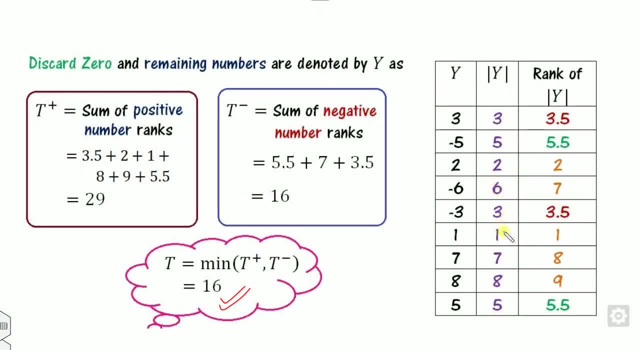 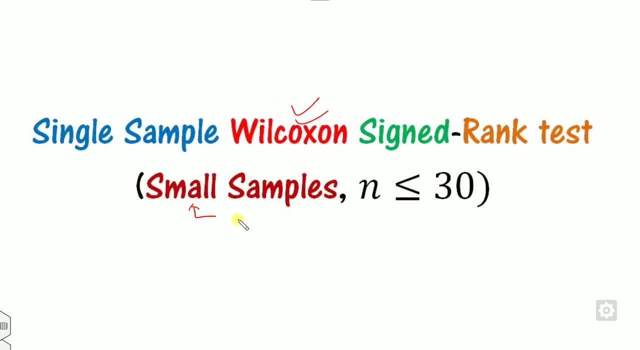 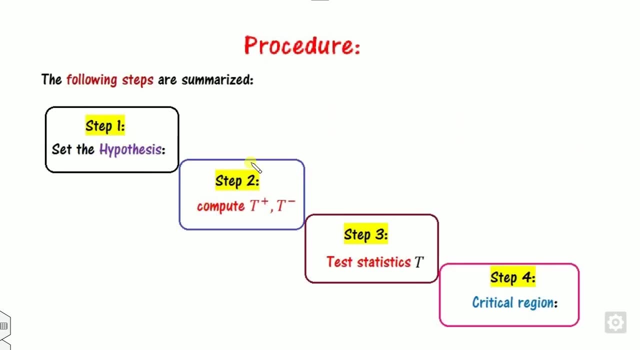 You have to take care that, whether it's a, any number are repeated or not. Now we will start with the Wilkerson signed test piece. So first one is a small sample. So the sample is said to be small when the sample size is less than or equal to 30.. 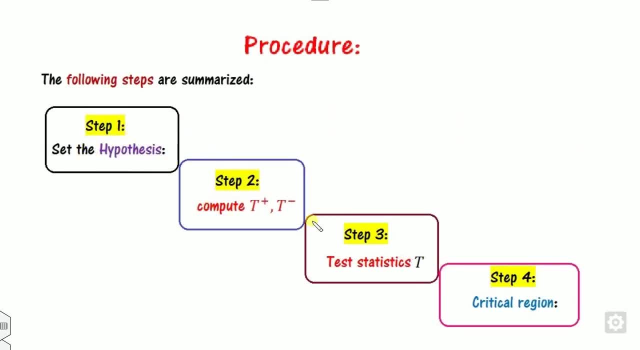 So I just discretize this into the four step. This is the same as that of the previous lecture. We define the null hypothesis and the alternative hypothesis, How we compute the T positive and T negative, as we discussed in the previous slides. We have to firstly use the signed rank. 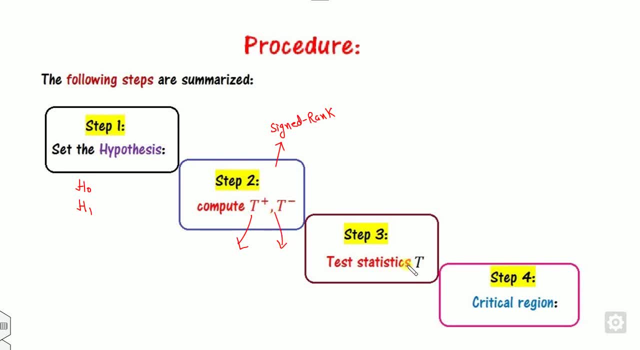 And then we will calculate the T positive and T negative. Then step number three, how to calculate the capital days. You have to take the minimum of T positive and T negative And then, finally, we use the critical reason. So we will define the step one- null hypothesis- as equal. 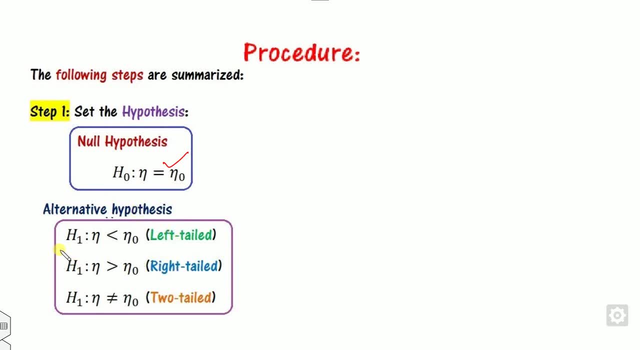 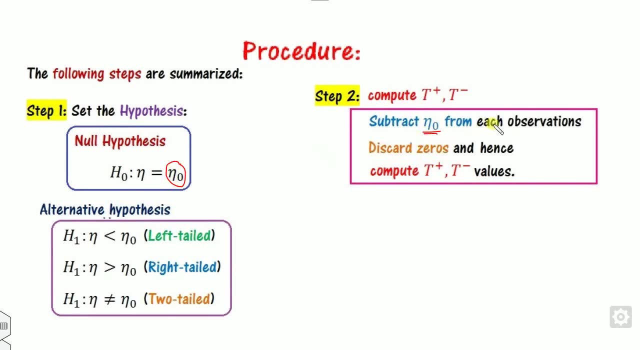 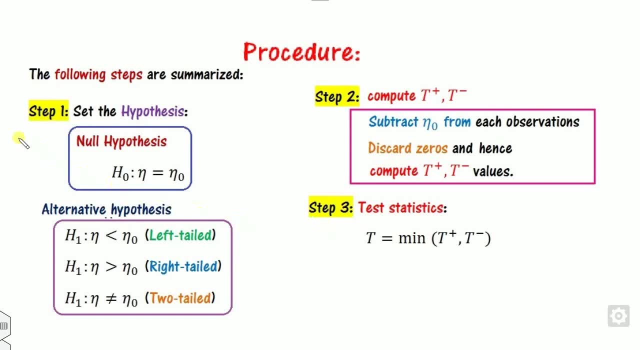 And then step number four, null hypothesis as equality Alternative. are either of them based on the quotient? We will subtract this number, whatever you have written here, from the each, Then we will compute the positive and the negative, Then we will calculate the minimum. 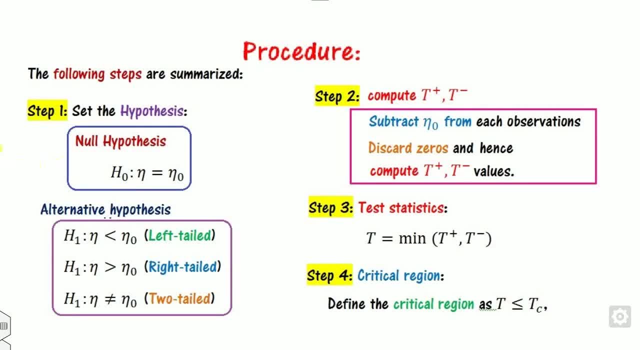 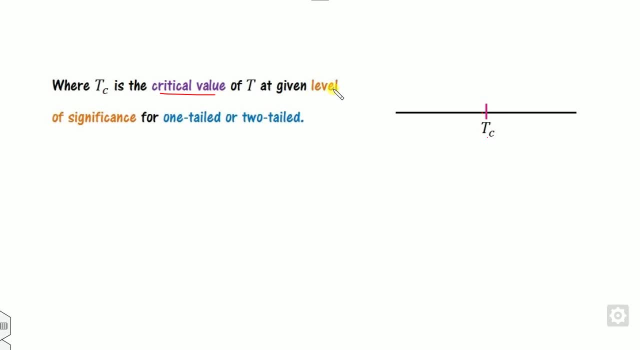 And we will check the critical value. And this is the quotient. So what is the Tc? Tc is nothing but my critical value at here And this is the value at given level of the significance Once you will get, then we will define the critical reason. 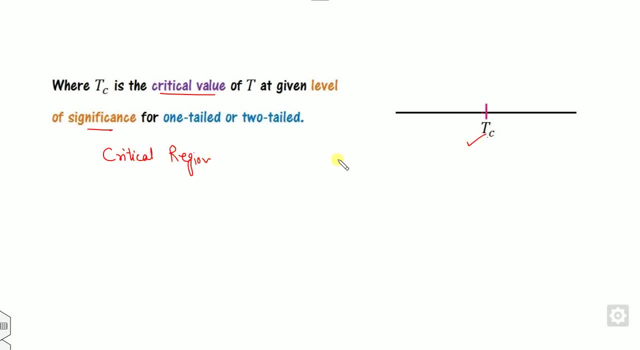 Corresponding to this value of Tc. How you define the critical reason is this number. So this is So the critical. You can say the critical reason is less than equal to Tc, Then we will check that. what is the value we obtained from the step three of the capital day? 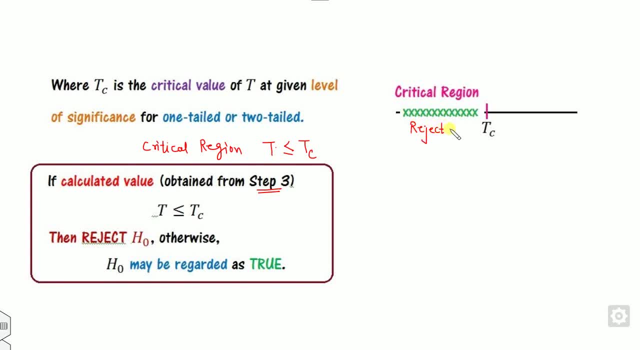 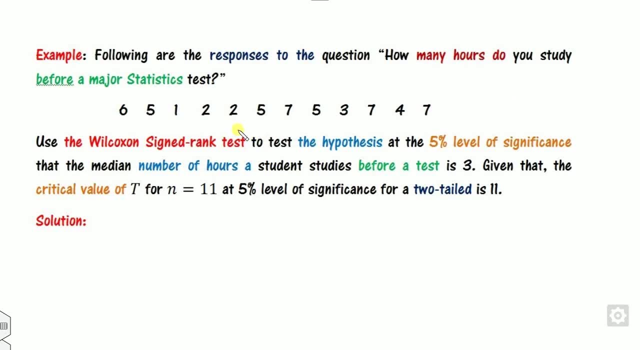 If it lies in this reason, We will reject H0.. If it lies in this reason, We will accept H0.. Here is minus infinity, Here is plus infinity. So look at the example. If you remember the last lecture, This is the same example I have considered here. 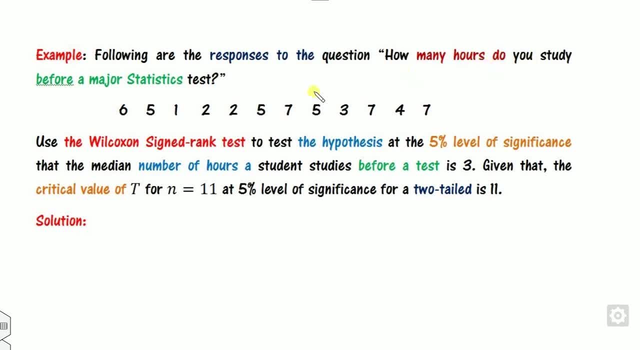 So following are the responses to the quotient: How many hours do you study before the major statistics test? So firstly, we will define the step one, Define the null hypothesis And define here. So what do you want to claim? So look at the median. 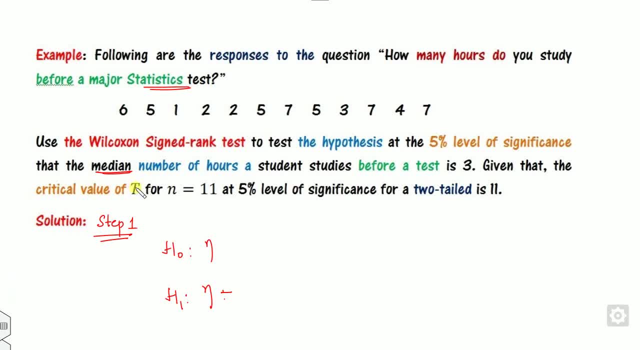 So your target is to calculate the median Of the student before the test is 3.. So that is the is, That is the equality. So that is always be a here. So it means this is opposite to each other. So this is means equality. 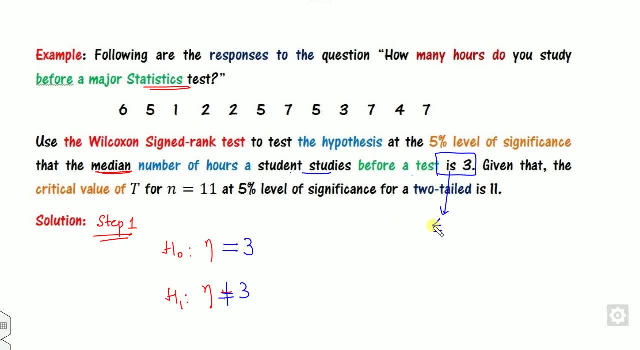 So this is H0.. If this is be like, say, less than of 3 or greater than, Then we have to define H1.. So this is not equal to, So it's a 210.. Now for the step two. We have to compute. 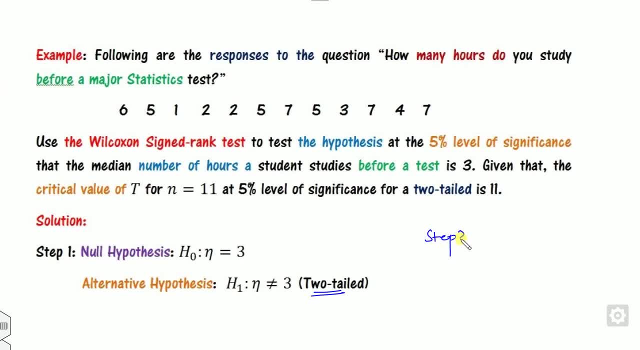 What is my step two is Compute T positive and T negative. How to compute them? Look at, this is a 3. So we subtract 3 from the each number. So this is my 3.. Then 2.. Then minus of 2.. 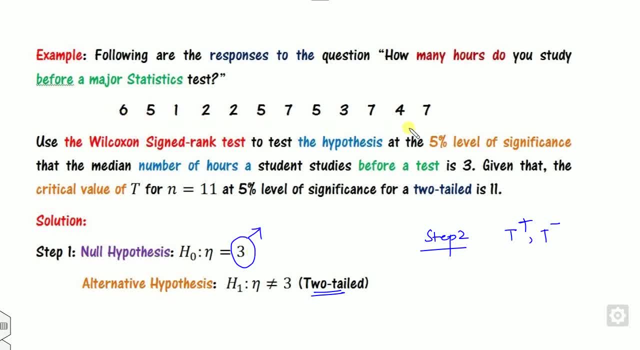 Then minus 1. And so on. So if there is any 0. Then you can discard them And the remaining entries can be represented as a Y. Then take a look at this. So this is H1.. This is H2.. 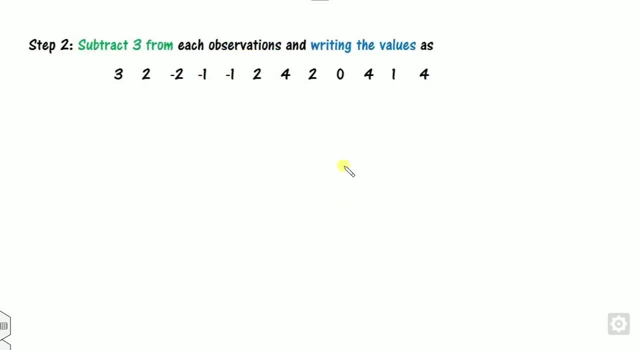 This is H3.. This is H4.. This is H5.. This is H6.. This is H7.. This is H8.. This is H9.. This is H10.. This is H11.. This is H12.. This is H11. 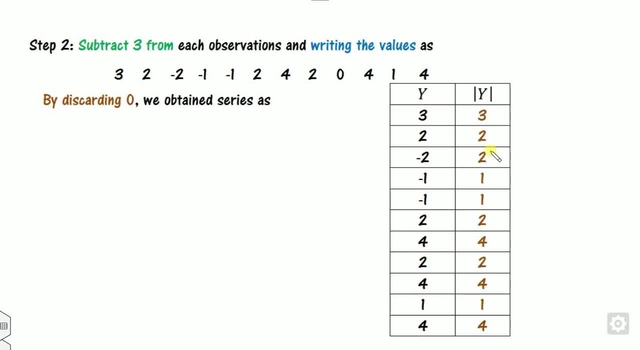 This is H12.. And you can take, here you can Genome, This is Genome Here, Genome here X by Genome. Now Genome can look for y, Y. Then take as a mod 근� here Now you can rank them. 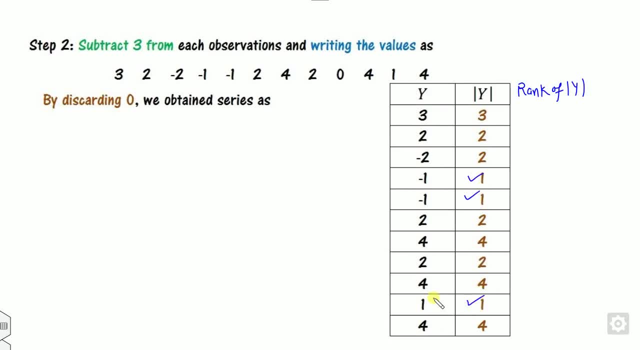 So how you rank them? So take the smallest number, 1.. But one occurring three times. So this is the position 1,, 2, and 3.. So you have to take 1 plus 2 plus 3 divided by 3.. 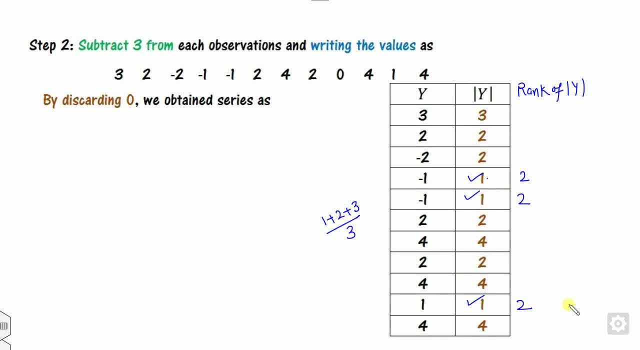 So what is that? Two? So you have to put two against each number. Look at that Now. what is that next number is Here? 2, 3 times 4 times. so what is that number is? this is a 3 already gone, so this number is 4. 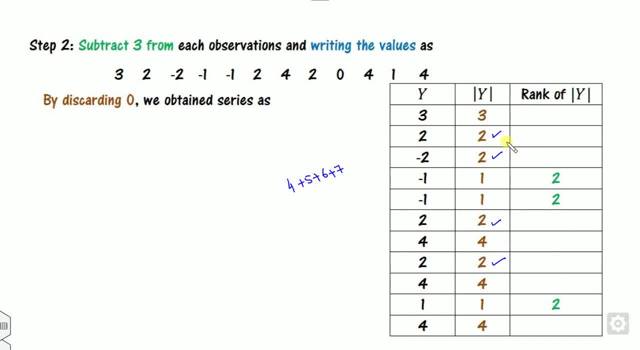 5, 6, 7, because they are 4 times. look at: 1, 2, 3 is already there- 4, 5, 6, 7 divided by 4. so what you get is this is my 23 divide- sorry- 22 divided by 4, so it is 5.5. so look at, that number is here. 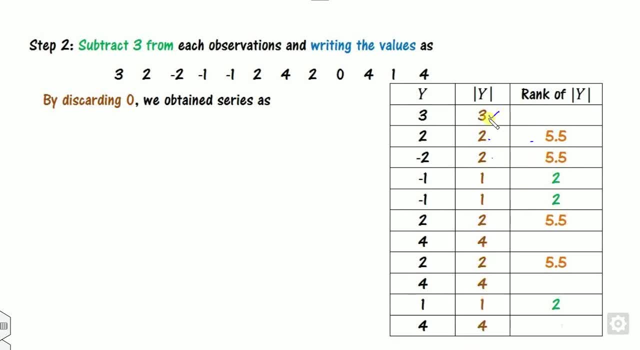 now, after that, the smallest number is 3 and it appears only one time. so what is the rank is how many numbers we have put up: 1, 2, 3, 4, 5, 6, 7. now it's a 8, after that 4 appears. 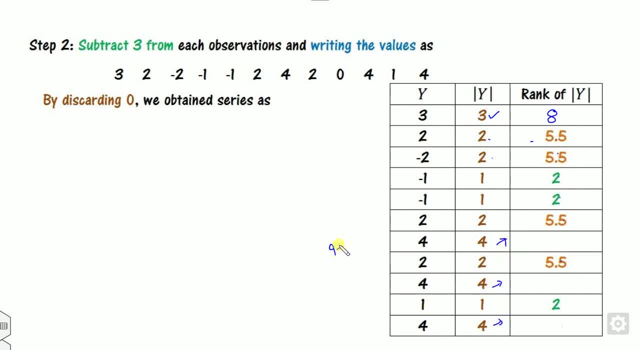 3 times, so that now numbers are 9, 10 and 11. so you have to put here: okay, so you will get the number as my 10, 10 and 10 once you compute the rank of this. then you will get the number as my 10, 10 and 10 once you compute the rank of this. 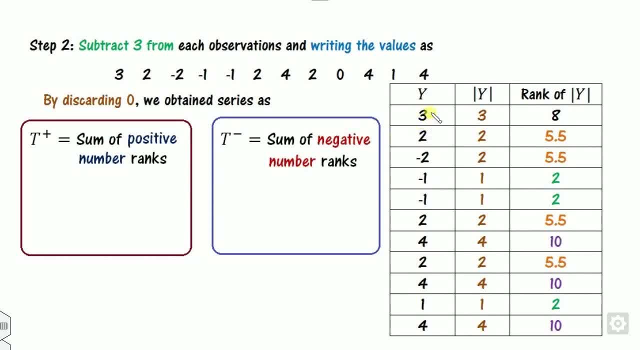 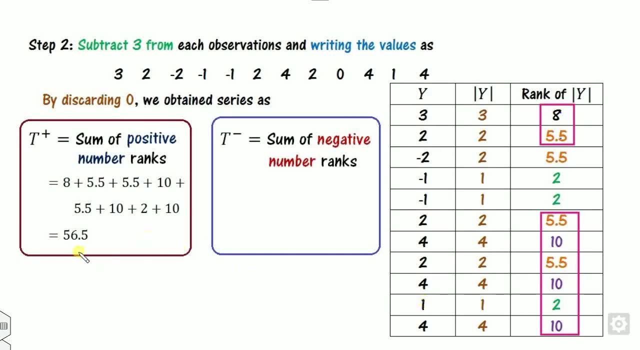 then we will define the t positive and t negative. what is the t positive? is these two numbers, and these four are there. the corresponding ranks are this and the first two. so this will be my look at that: 8, 5.5 and then. so this is here. what is the t negative? is this number, this, this or you? 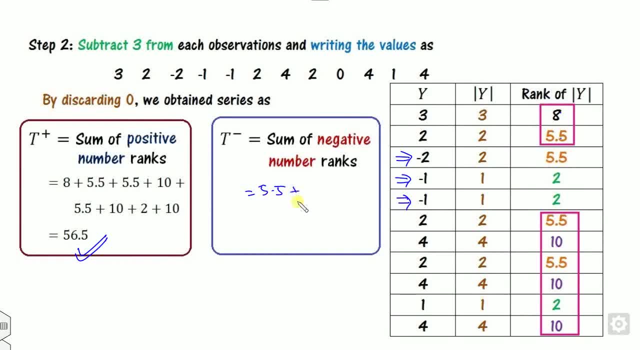 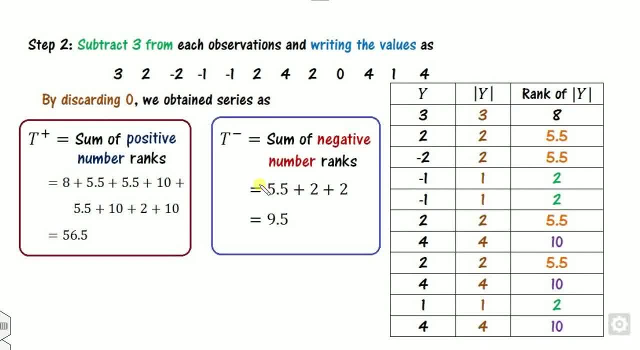 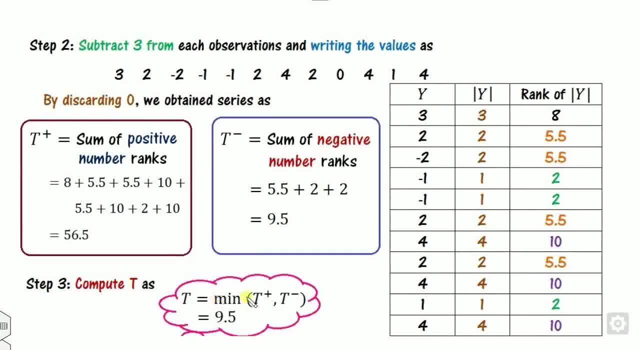 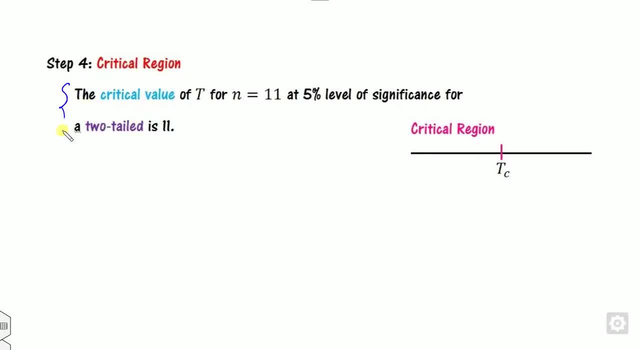 as 9.5, as my t negative, then this is step 2. then you have to define the step 3. that is the minimum of this you will get as a 9.5. now look at that. you need the critical. this value is given to you in. 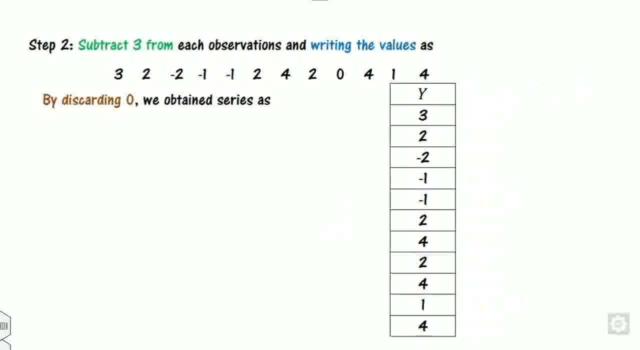 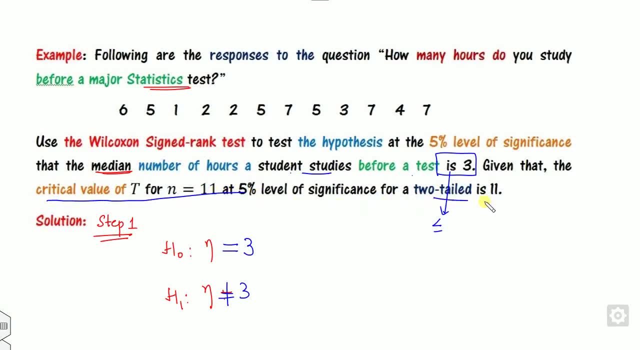 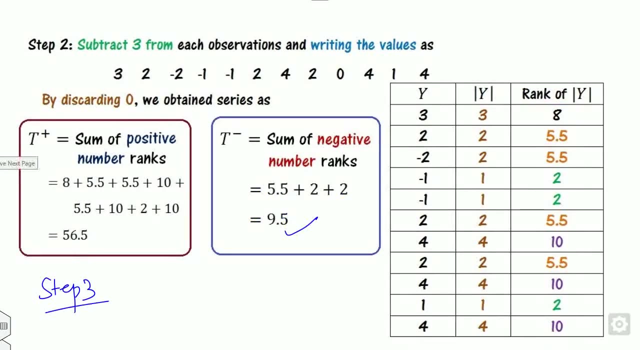 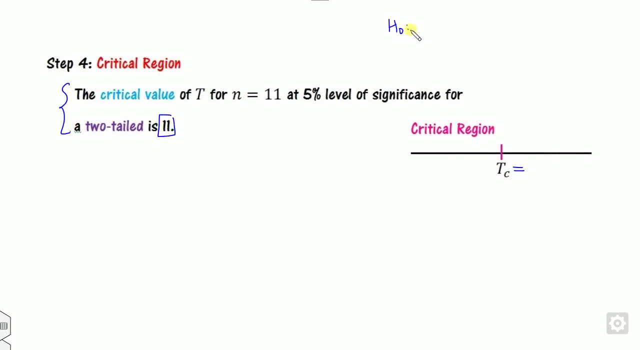 the statement. if you look at that, the values are given to you in the statement. look at the last and critical value of this: at n is equal to, 11 is 11.. 11 again, so you can compute them. step number four. so this value is given to be as a 11. look at that. what is my? h0 is here, h1 is not equal to, so it's. 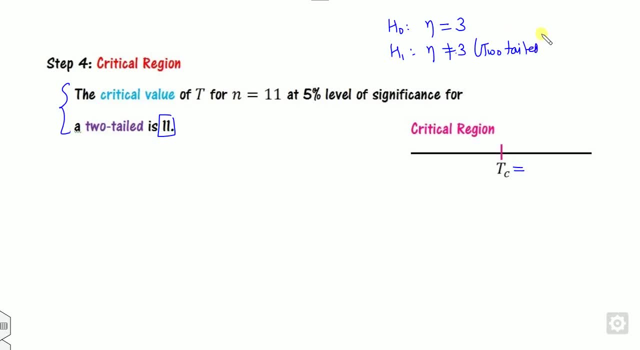 not equal. it means this is my two tail. so if it is two tail, that value is given as a 11. so what is that? this is my critical reason. so you have to write: t is less than 11.. so what is the value of that capital? t we obtained in the step 3 is 9.5, so 9.5 less than 11. so it. 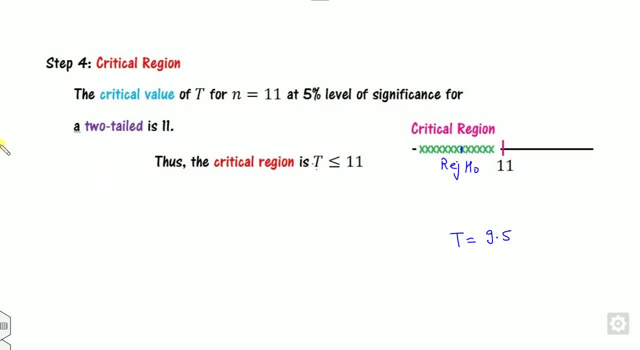 lies here. so what is the meaning? is we reject at 0 now, since this value is less than 11, so we rejected h0. what is your h0? is eta is 3. this is not equal to 3, so it means this is rejected. so it means this one is accepted. so what is the meaning is the test is not equal to 3. 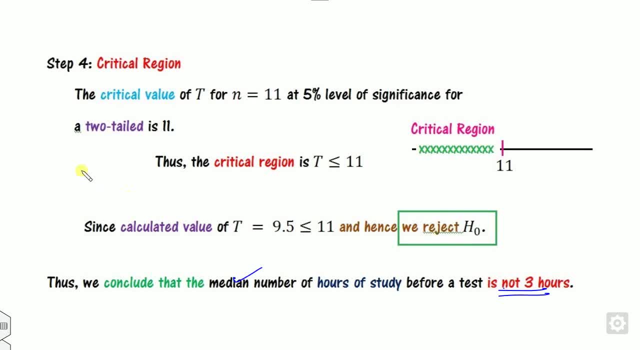 the median number of the hours taken before the test is not 3. okay, so if you remember this, the same example we have discussed by using the sign test also, but in that sign test, if we apply both the sign test and they will constant test to the same. 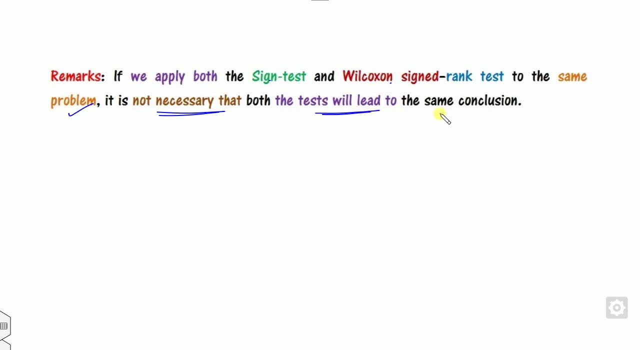 problem. it is not necessary that both the tests will lead to the same conclusion. for example, in this case we will we conclude that we reject at zero. can it be the same? it may or may not be. so we have done the same example, using a sign test, and we conclude that we will fail to reject. 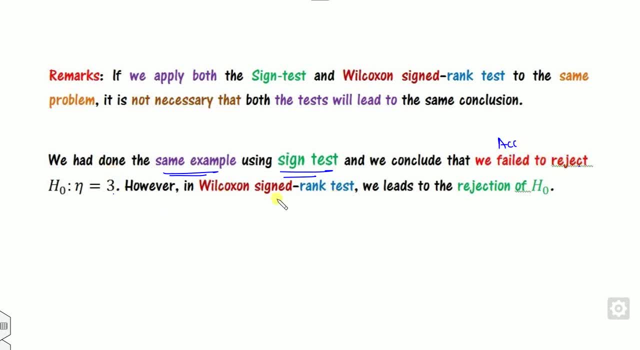 the h0 at here. however, the wilcalson sign test leads to the rejection of the h0. so which one is the better? obvious that the wilcalson sign test use the more information as compared to the sign. so the results computed through the wilcalson sign test will be a preferred one over the sign test. 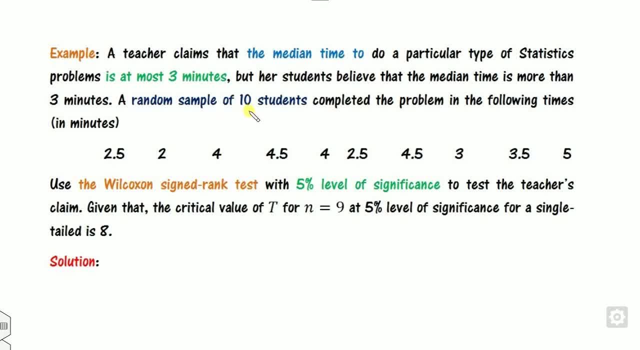 now quickly move on the second examples. these are again the same example we cover in the last sign test video. so what is your h0 and h1? so look at that. the particular type of the statistics problem is at the most three minutes, so you have to test. the teacher claim, so this: 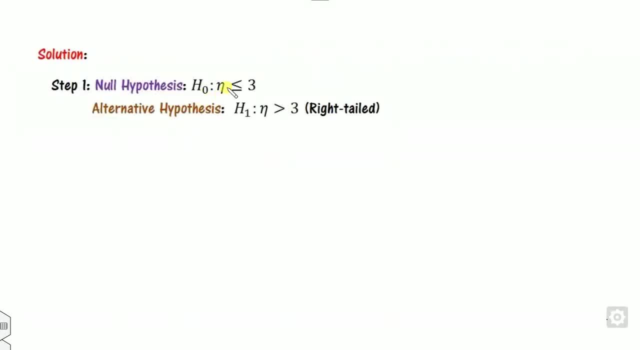 is the teacher claim. this is the at most three hours. so look at that, the at most three hours there. so this is my edge, because equality part will always be lies in the null hypothesis. opposite is here. so this is the right tell and if you think about that, look at that. this is a single. 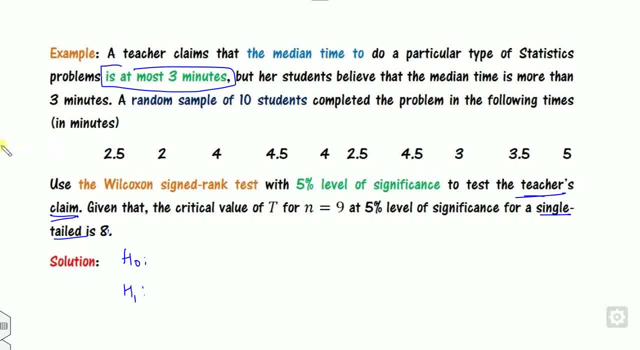 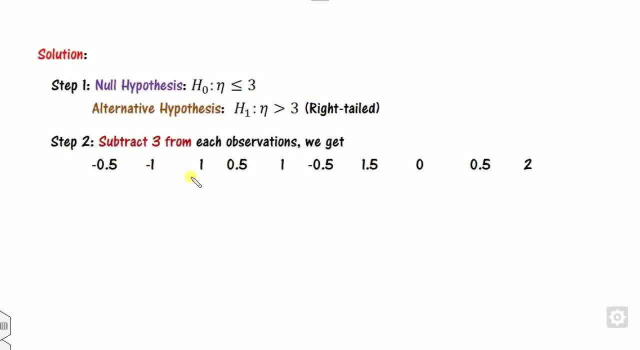 tail value given as a eight. now what is the step? number two is you have to subtract this number. this is three. so subtract three from each of the numbers you will get as here. now discard zero, if any. yes, this is one number, so you have to write this number as here. compute mode of y, you will get. 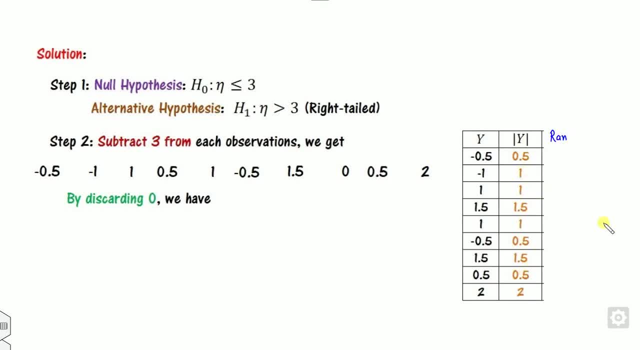 here now you can find the rank. so which is the rank? so we will do that here and we will now eat. smallest number is 0.5, 1, 2, 3. so 1 plus 2 plus 3 divided by 2, so you will get 2, 2 and 2. sorry, 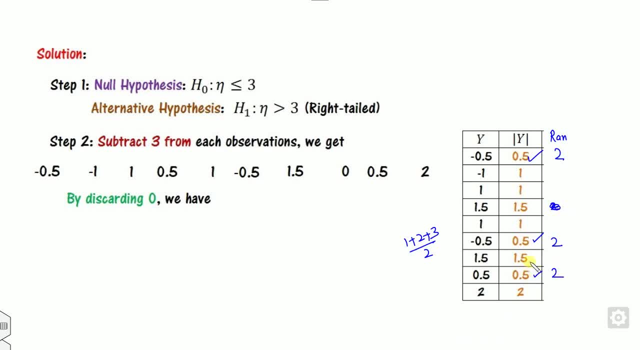 these are there. after that, the smallest number is 1. again it appears 3 times, so 3- position already already there. 4, 5 and 6 divided by sorry, it will be a 3, so 4, 5, 6 divided by 3, it's a 5. 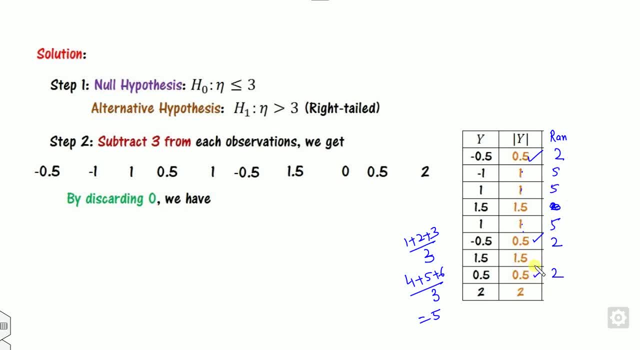 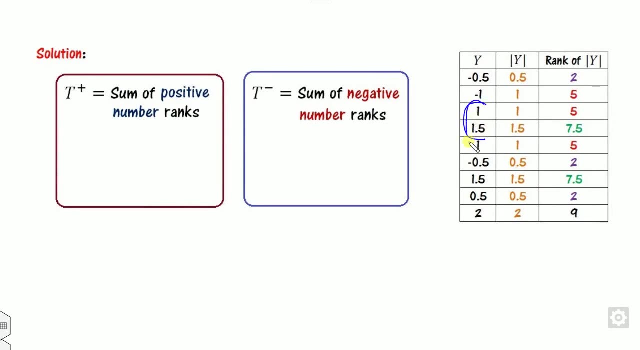 so this is 5, 5, 5, and next one is 1.5 and next one is here. so you will get these numbers now. in order to find this, you will find the t positive and t negative. so what are the t positive? these three numbers, and these three numbers are there. 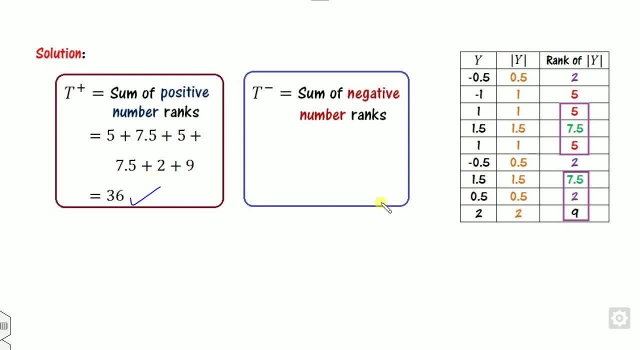 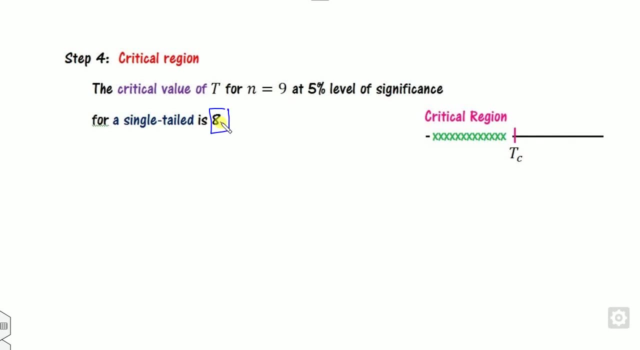 so you can compute them as this, as this, and the remaining are the t negative. now you can compute the t minimum of this. now you define the critical value. it is given to be a critical value 8 for the single tail, so this value is 8. find the critical reason. this is my. 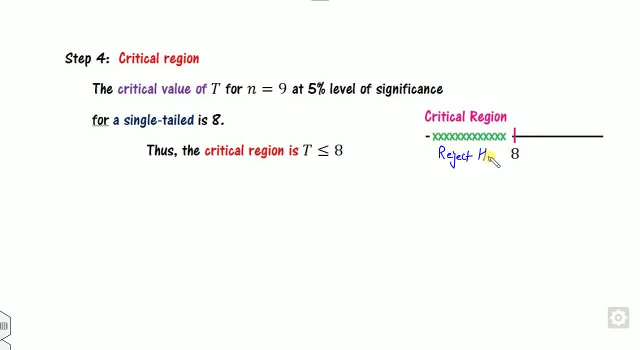 less than or equal to 0. now you can find the value of the t we computed. the step 3 is 9. so where it lies that it is not satisfied, 9 lies here. so we fail to reject h 0 at 5 percentage level of significance. hence, what is the h 0? is this is less than 3. h 1 is greater than 3. 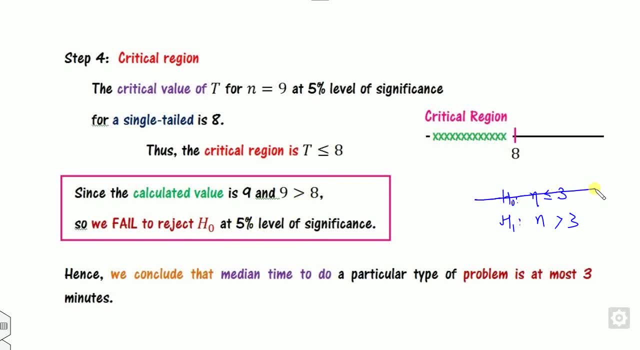 so h 0 is rejected. so we will reject this. no, sorry, it is greater than so. we will accept h 0, so it is accepted. so it means the median time is, at most 3 is valid. look at one more example related to the large sample. 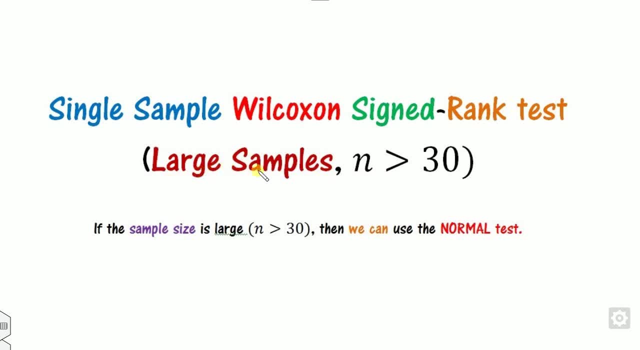 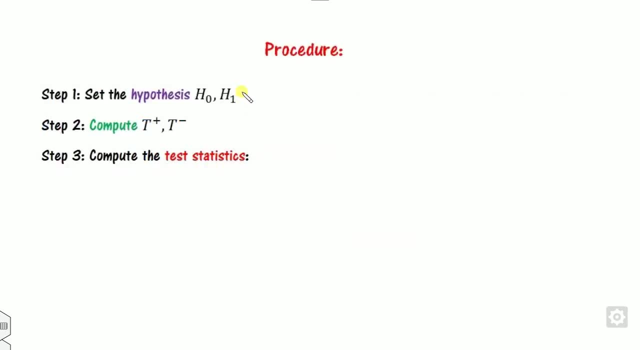 so how you solve the problem: when the population size, when the sample size is greater than 30, then we call as the large sample. so how the procedure are same. firstly, we define h 0 and h 1, we compute the t positive and t negative, same. the only change here is step 3. we will use the 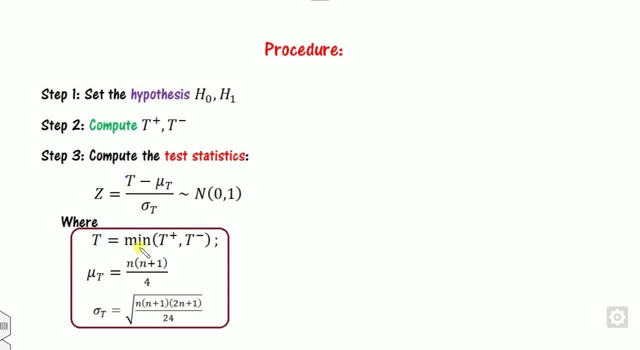 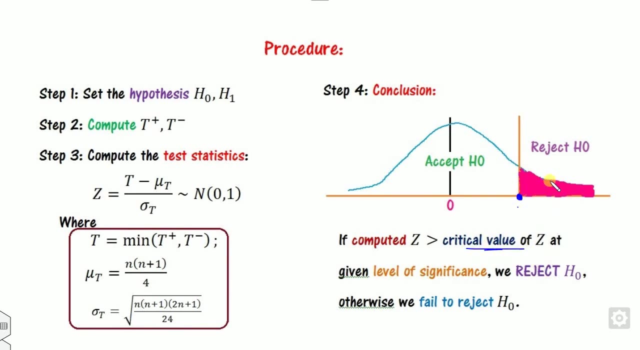 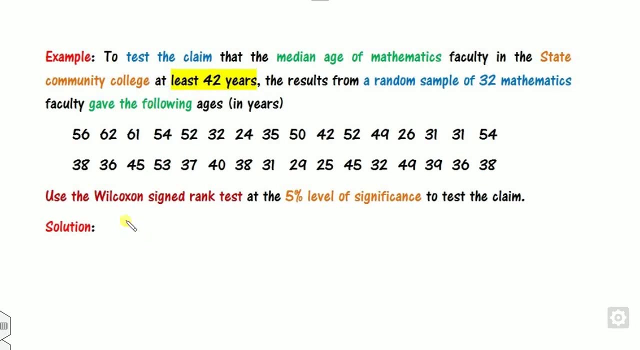 normal distribution. so normal distribution here. what is the capital? t same mu is the mean which is calculated as here. sigma is this, once you are finding this, which comes to be the final set. this have to be form, holy mass. it comes to be the final set here. so if we take h 0, then reward plus k. this is equal to maximum value only. so, with the help, 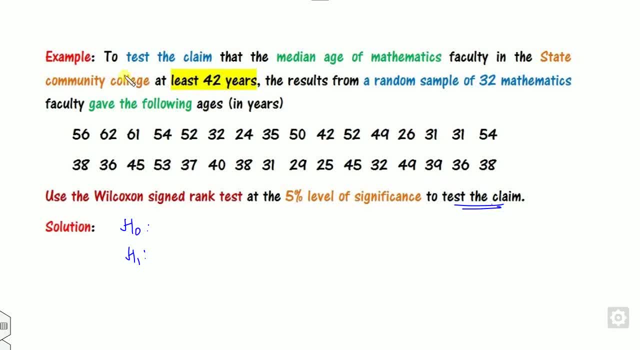 of total t and x minus minus t. faisley, we can only weird. all the sitting values there is that, which is that the limit value in this with respect to the value of two null, two point five, the value of igniter value of zip is equal to Desert value. that means it is at least 42. so what do we Kryden? so 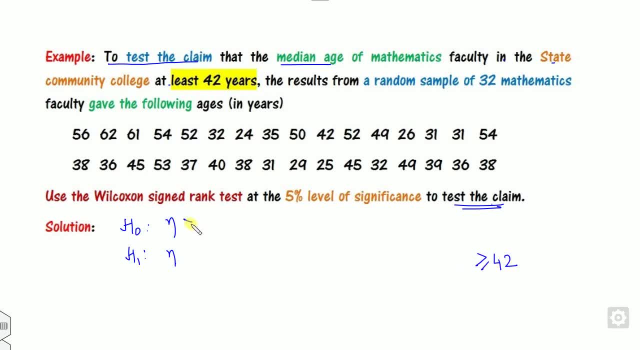 greater than or equality. so since it is equality, so this is my here. so what is opposite is 42. so this is null hypothesis. this is my alternative. so it is a less than it is a left hand. so what you can do is subtract 42 from each of the number. so 56 minus 42 is my 14, 62 minus 40 is my 20. 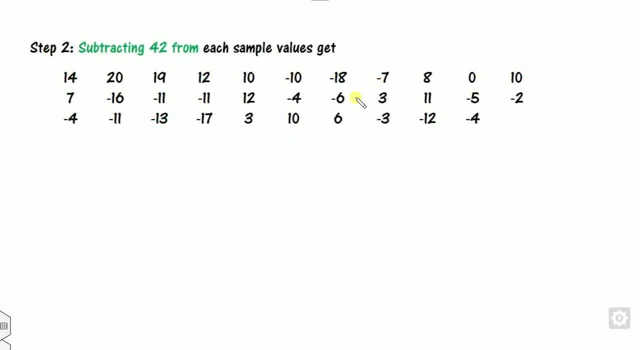 and so on. okay, now you can discard the zero and write all those numbers in terms of the y. so since the numbers are very large, so it is very difficult to write here, so i can represent this number here in the increasing order or you can write as such. 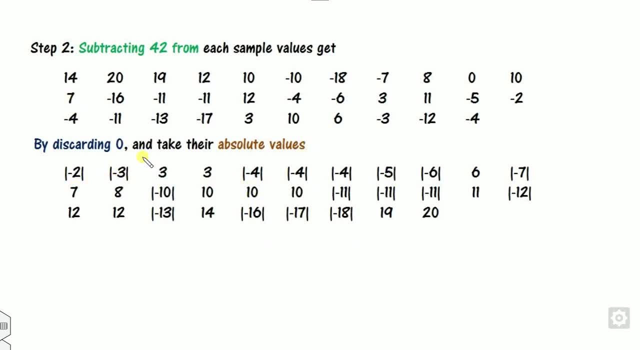 but i have right here in the increasing order. so what is that increasing order in their absolute value? look at that mod of two, then three and then so on. now we can rank them, you, how you rank them. this is the smallest number in magnitude. so this is one. look at that. these are. 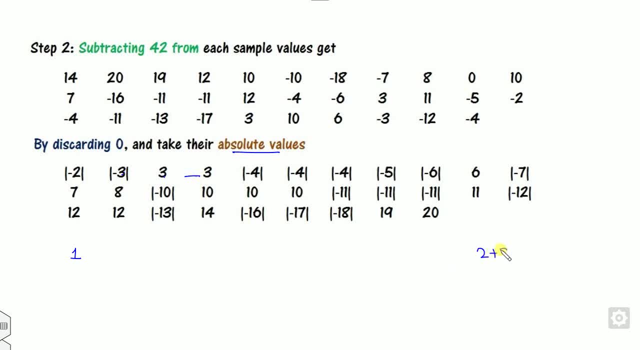 the same number. so this is the second, third and fourth. so how you rank them: two, three, four divided by three, so it is three, are the same number. okay, so we will rank them as here. now. look at: these numbers are same. so how many numbers we put up one, two, three, four, so it will be five, six and seven. 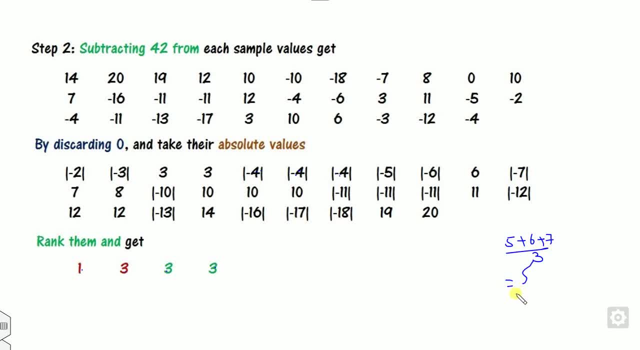 five, six, seven divided by, divided by 3.. So what is that? 18 divided by 3 is 6.. So we put 6,, 6 and 6 here. Look at, and similarly you can find here I use the two colors here This green color is represent for only those. 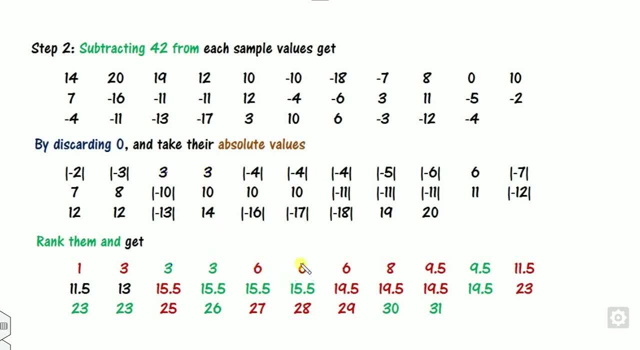 number, which are positive numbers, and this brown color or red color is represent for my negative colors. are there- Look at that- Everywhere where the positive numbers it appears as my green and so on. Now, once you are rank them, you will calculate the T positive and T negative. So 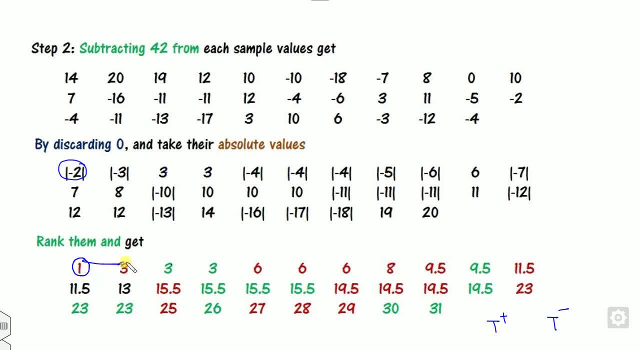 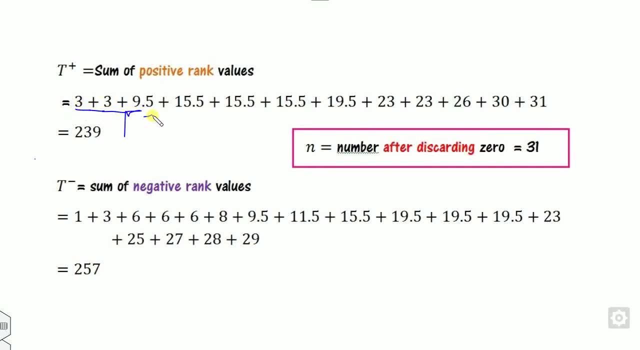 look at that, This number is negative. So this part, this part, okay, and so on. So all those colors which are representing as a green color is corresponding to my T positive. So we will calculate this. Look at 3 plus 3 plus 9.5 and so on: is my number corresponding to my? look at that. 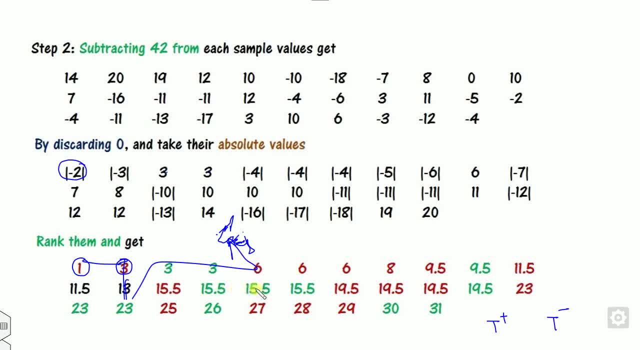 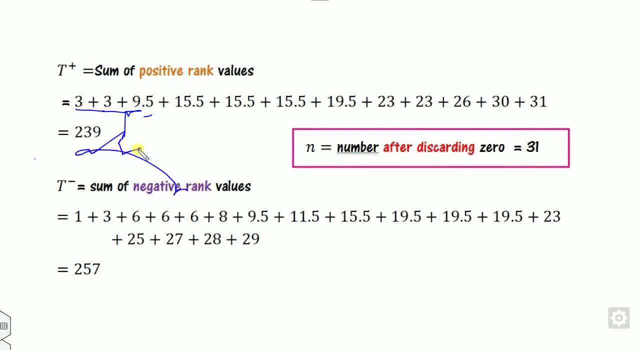 3, 3,, 9.5.. 15.5,, 15.5, all are my T positive, So you will get as this number. After that, you will calculate it T negative. This as my here, This is same. Once you will complete this, you will calculate the T. 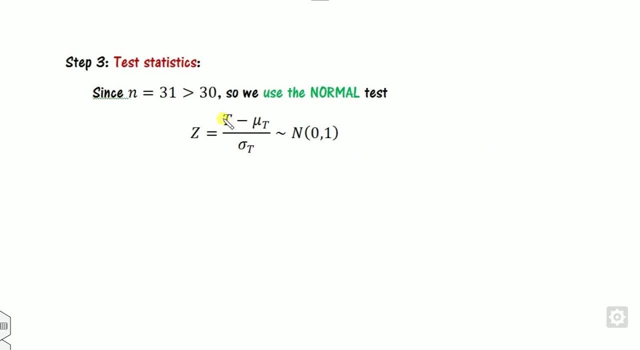 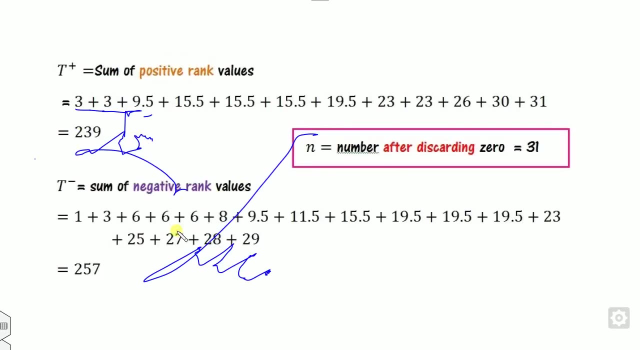 here my step term. So in this, firstly, we will see what is the formula for here. Now, what is the N? Look at that. In this case, what is the N is Number of the dice discarding the zero. So look at that. You have to rank this. 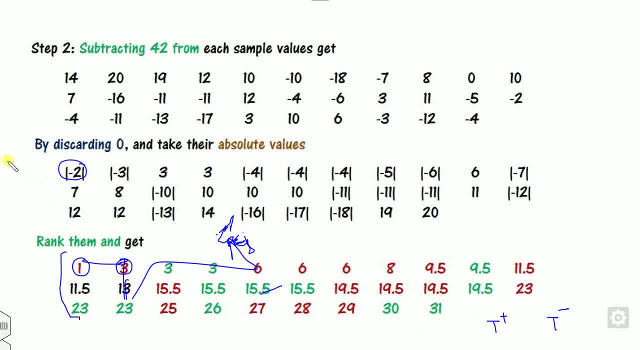 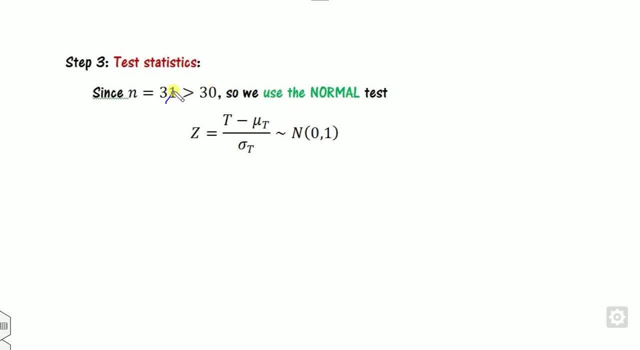 number. So how many numbers are there? This is 31.. So N is my 31,, which is greater than 30. So we use the normal test. If this N here, if N is my, say, 29,, which is less than of the 30,, then we will. 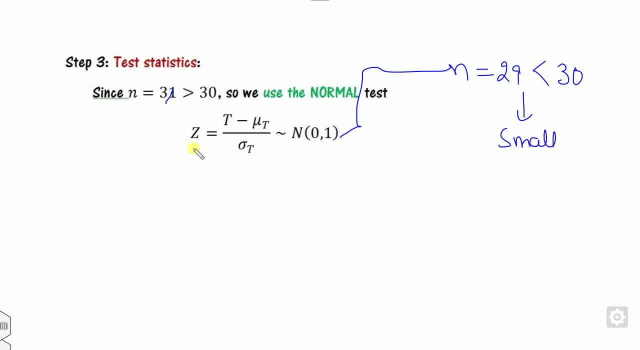 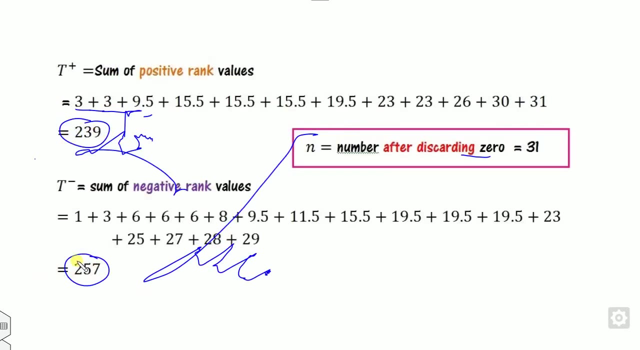 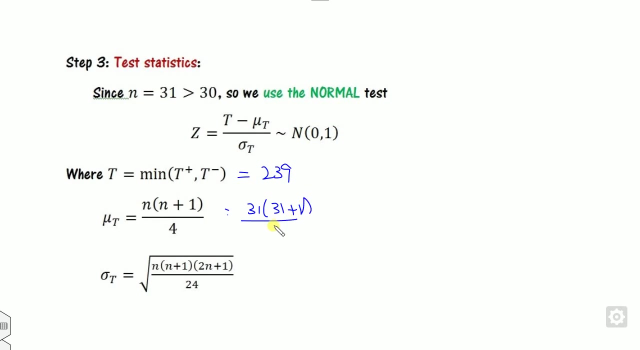 use the small test, as we discussed in the previous one, So we will calculate this. So what is that? T positive and T negatives? We have calculated 239, 257.. The minimum is 239.. N is my 31.. This and so. 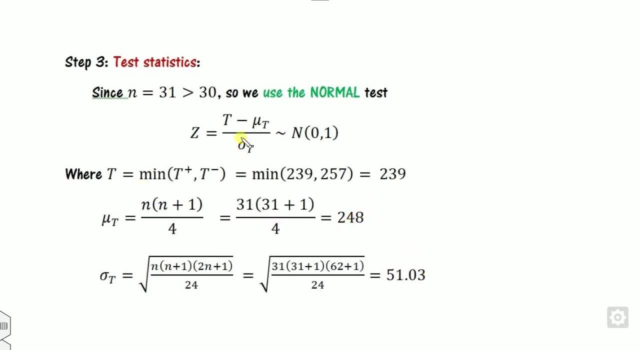 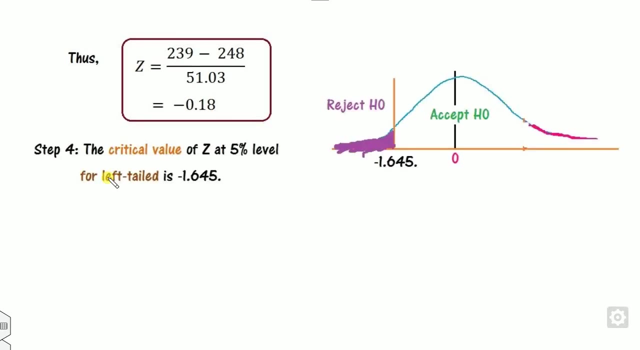 on. So we will calculate here. So once we will substitute this value in here, you will get 239 minus 248 divided by 51.03.. So what you conclude is here. So that is my step three. Now what is the step four? 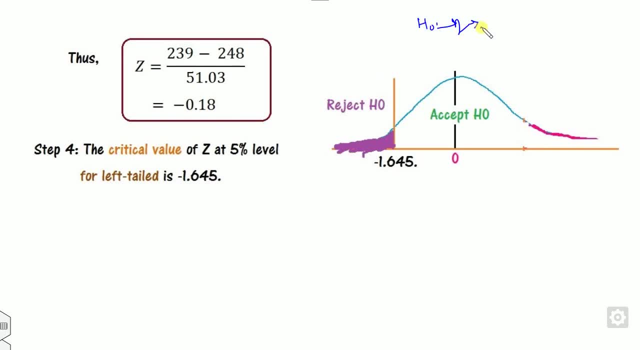 You have to. what is your H0 is? Look at that. This is greater than equal to 42 and H1 is less than 42. So since this is less than so, I have used here as my less than sign. Now, what is the?